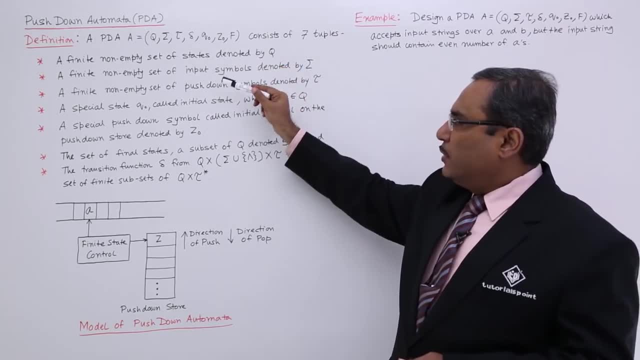 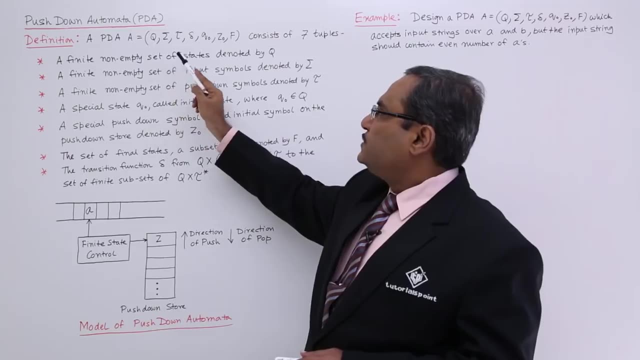 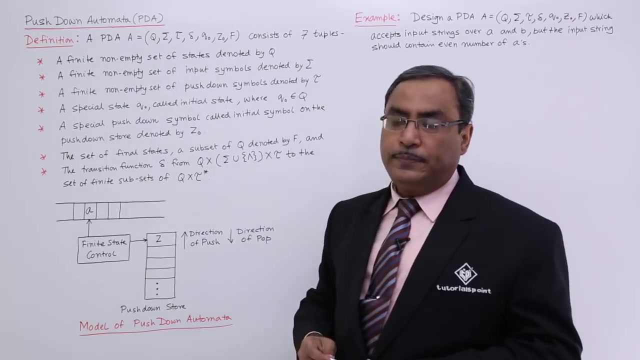 consists of seven tuples where each and every symbol we have discussed here, each and every symbol, So now see a finite, non-empty set of states denoted by Q. So Q will be containing set of states and that is finite and non-empty. A finite, non-empty set of input, symbols or input. 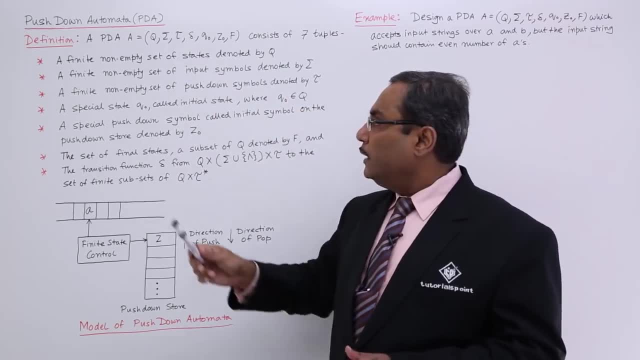 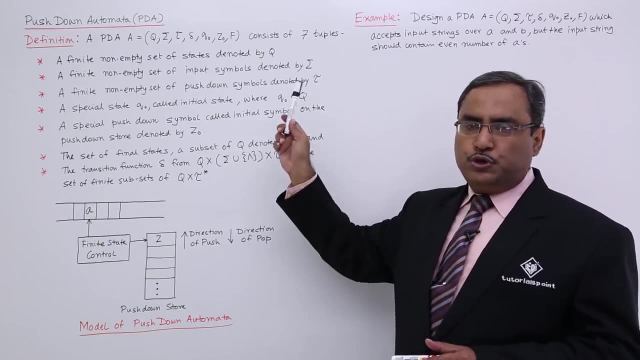 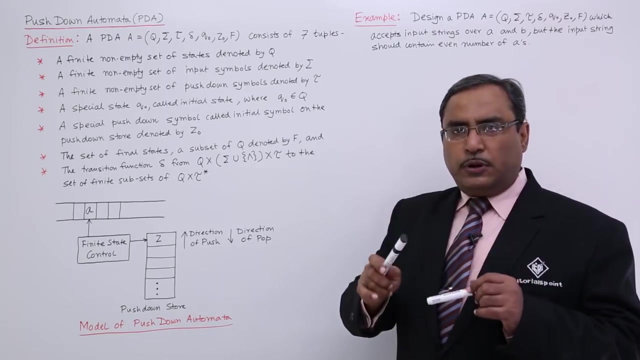 alphabets, denoted by sigma, A finite, non-empty set of push-down symbols, denoted by tau. In our push-down automata there will be one store, the push-down store, one kind of stack, So all the symbols which we can push there or we can pop. 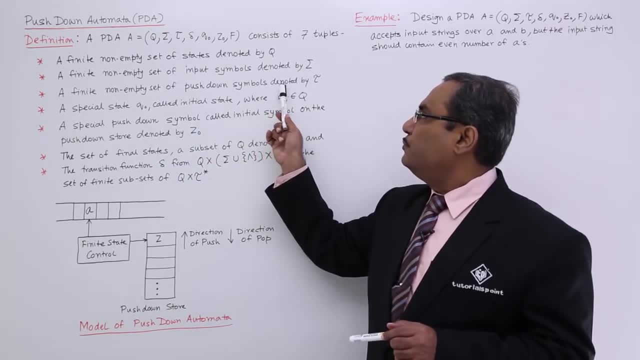 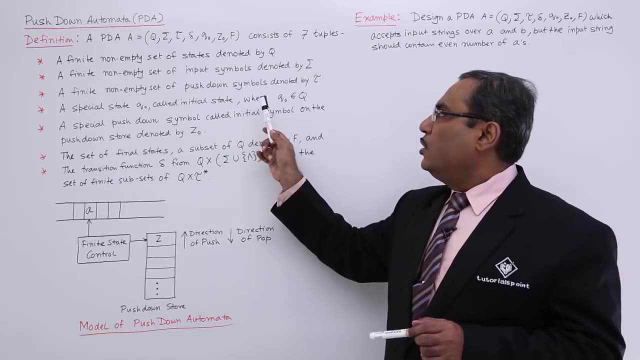 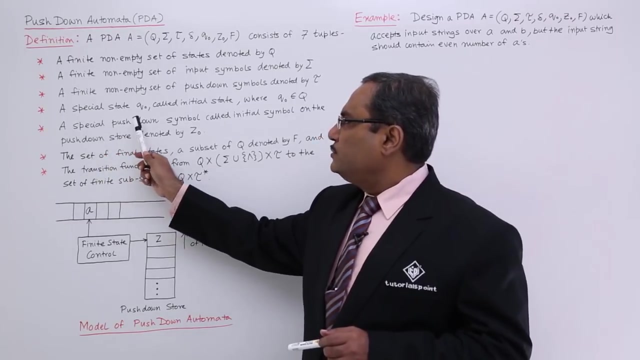 from there will be kept in this particular push-down store symbol set that is my tau. A special state, Q0, called the initial state where Q0 belongs to capital Q. set of states that is the capital Q. A special push-down symbol called initial symbol on the push-down store. 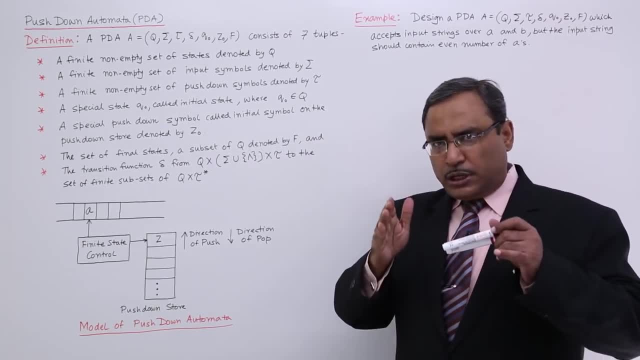 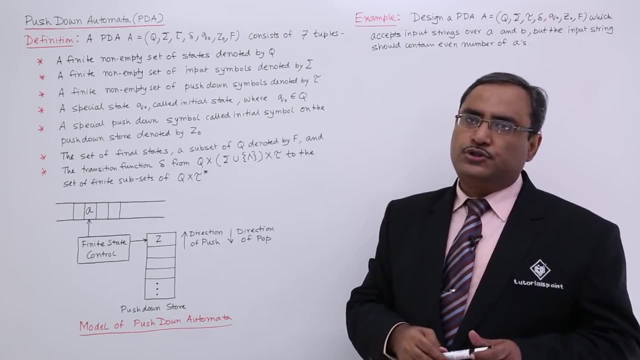 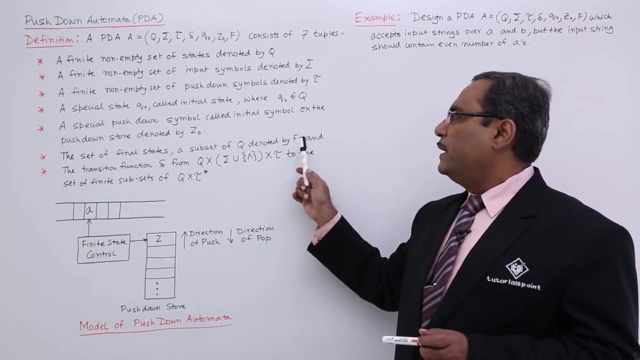 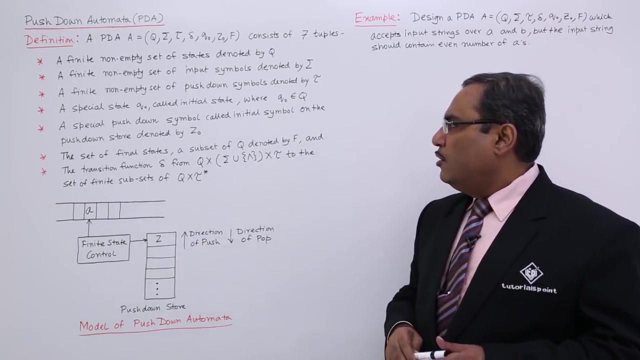 denoted by PDA. So initially you shall consider that the push-down store symbol Z0 will be at the top of the push-down store. you should consider that one, The set of final states, a subset of Q denoted by F. So F is a subset of Q and the transition function delta from Q cross. sigma union kappa cross tau to this is Z0.. You should consider that is a setup to draw in capital K code, that is R 1 plus 1.. Each time you draw each of these vectors get 1 plus 1.்F cyc of. 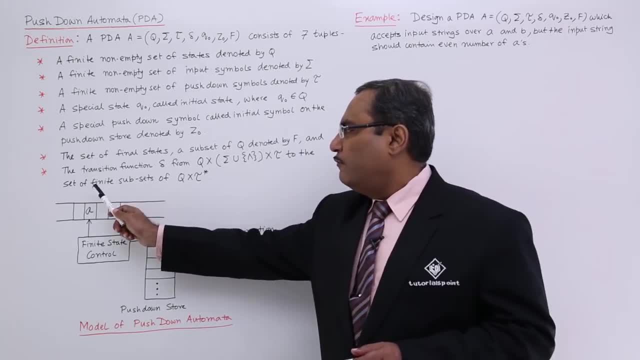 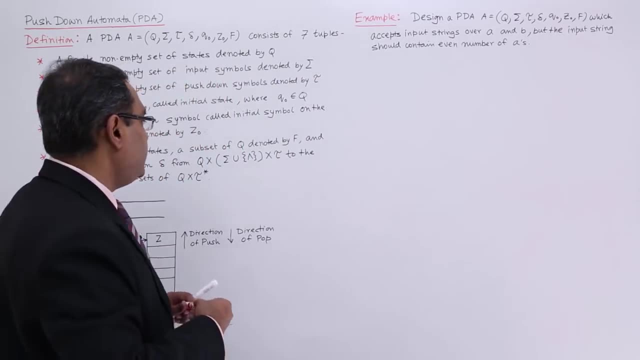 不是 mod if P garbageême actually railroad vanishes into overlook. That means this: make no reason to cross tau to the set of finite subsets of q cross tau star. That means it is telling that it is telling that q cross sigma union kappa cross tau. cross tau will map into q. 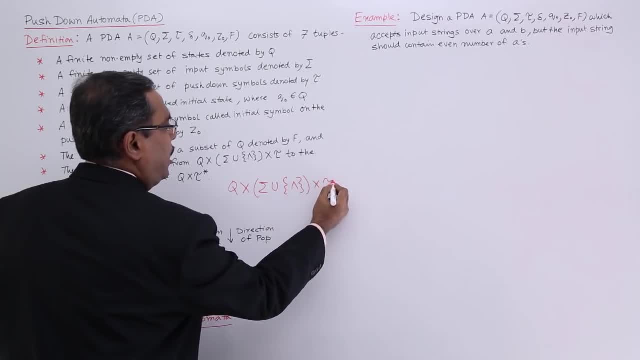 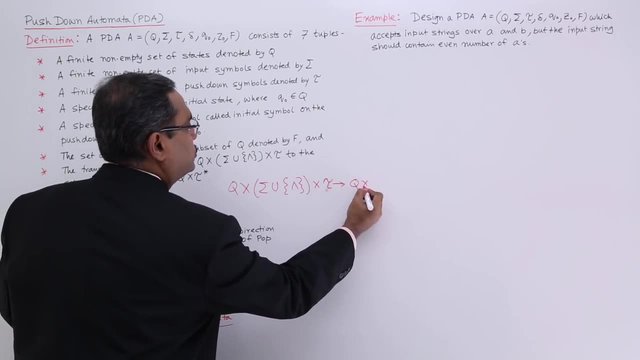 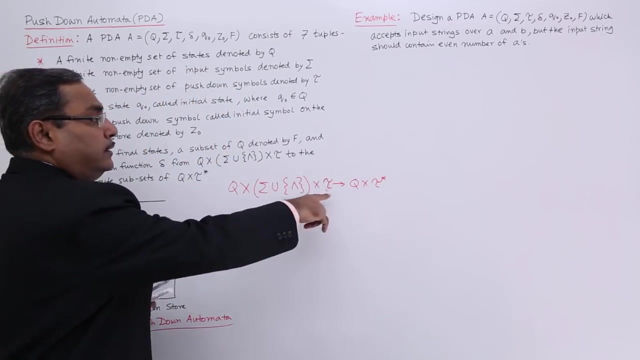 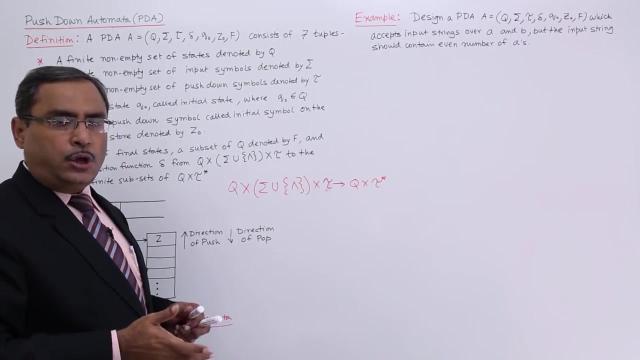 cross tau star will map into q cross tau star. So that is the, that is the, that is my delta. That means what is cross? cross means Cartesian product, means what? all possible combinations of this elements, this elements and this elements. So that is our. 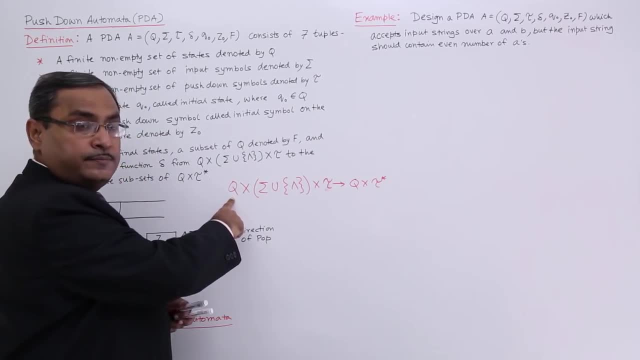 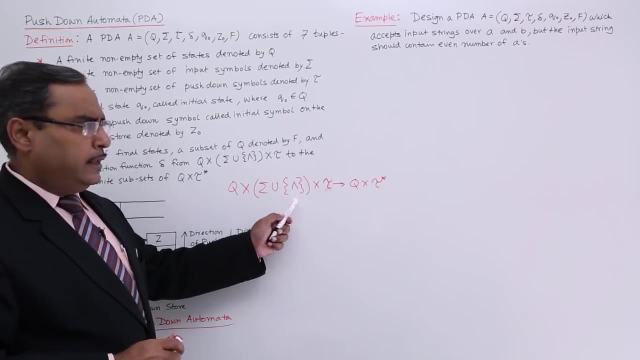 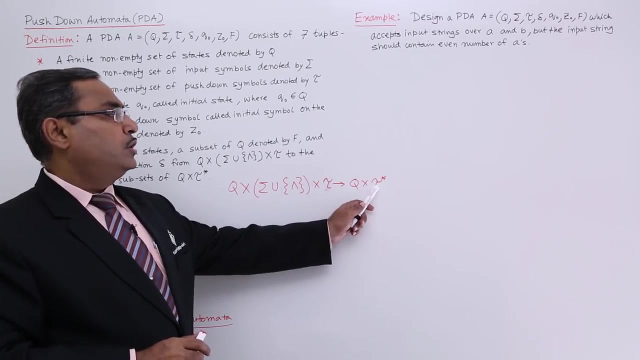 cross, So it will take one of the states. it will take one of the symbols from sigma. also it can consider kappa- and it will take one of the symbols from the pushdown store and which will map onto q cross, tau star, That means, which will map onto one of the 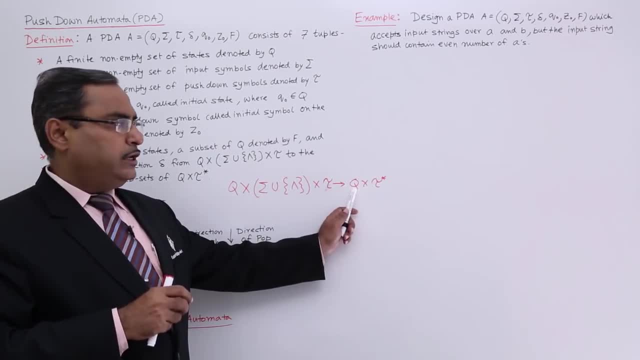 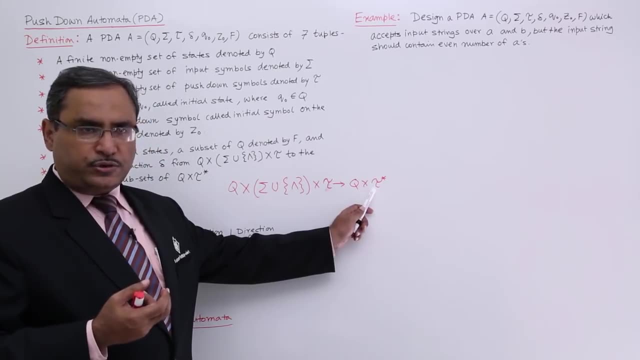 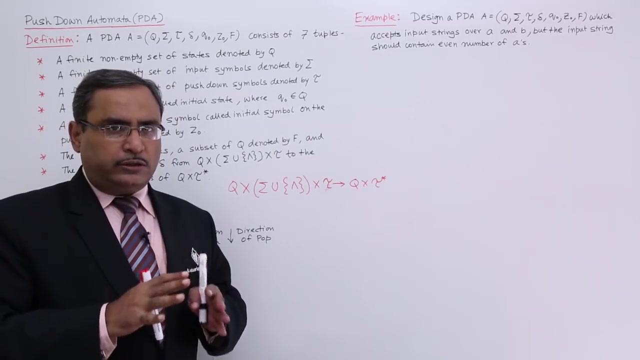 states in q and combination of one of the states in q and some set of that is the one, or more than one, or kappa null is also allowed because it is tau star. So in this way the delta has been defined. I think, if the conception is not clear up to this level, if you solve this problem, 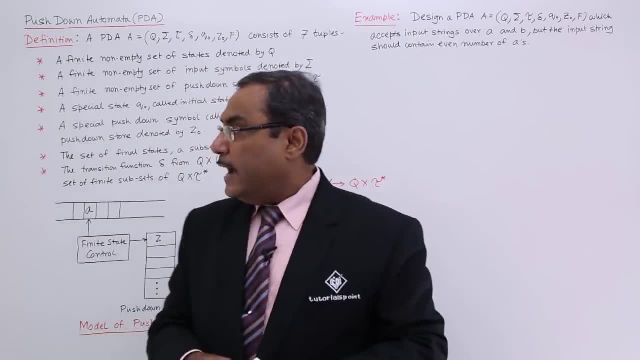 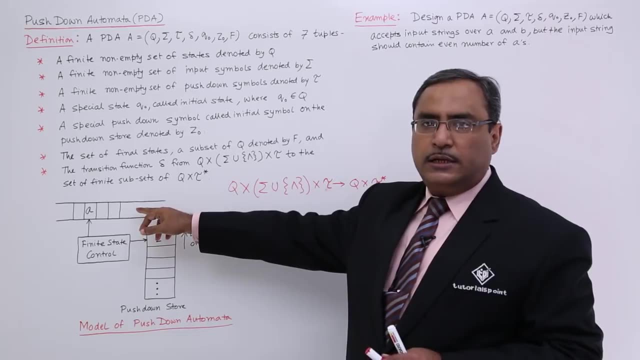 then everything will get clear to us. Now the final diagram is like this: we are having one tip and it is having. several cells are there and we are having some input symbols are there. So whatever the symbols you are finding here, they are nothing but belonging to sigma and 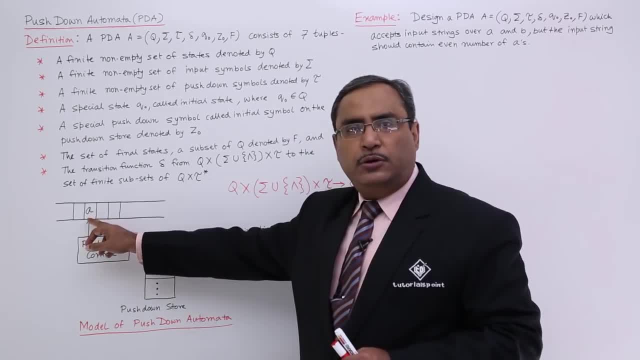 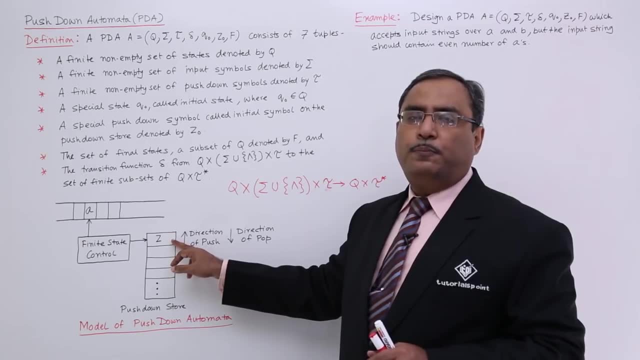 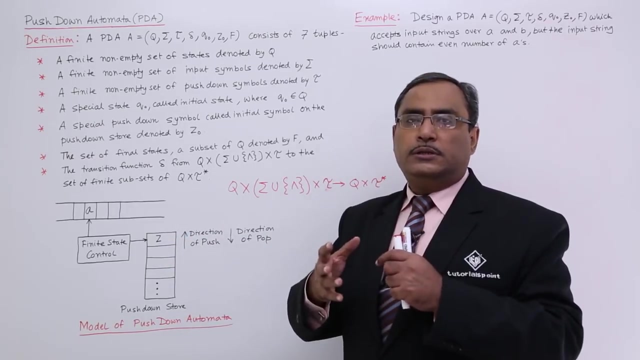 this is a finite state control, So it is pointing to this particular symbol rate from the input stream and also this is pointing to the one of the stacked symbols, or pushdown store symbols. This is known as a pushdown store, So initially it will be Z: 0 and if you go on pushing some other symbols, 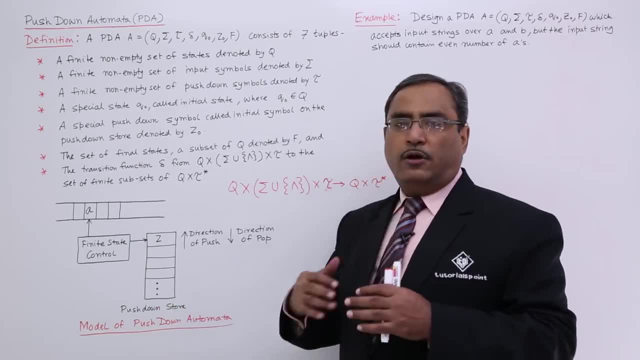 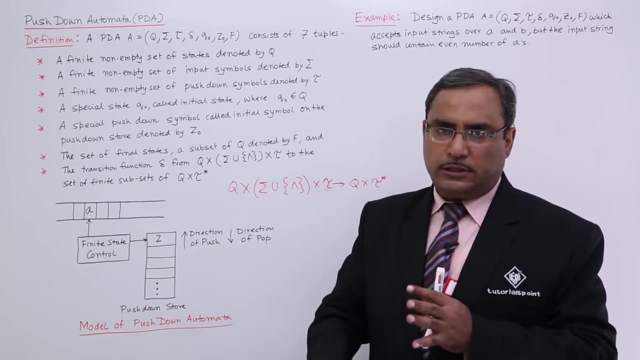 on the top of the stack, top of this particular pushdown store, then obviously that symbol will become that top most symbol and this finite control can read only the top most symbol, not any other symbols which are there in that, in theافice. So the control of the 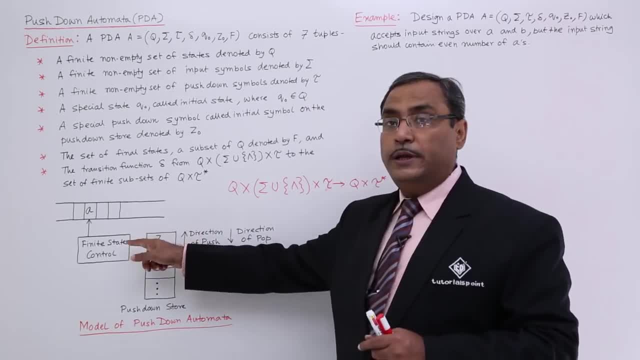 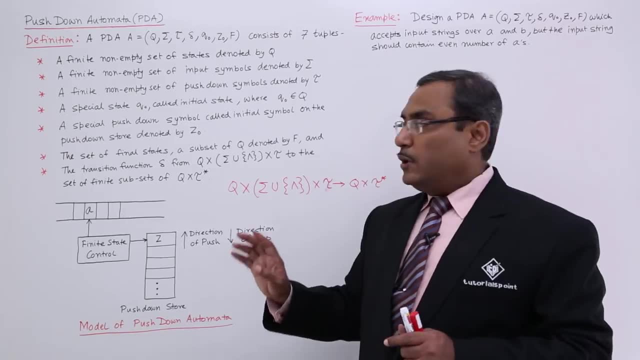 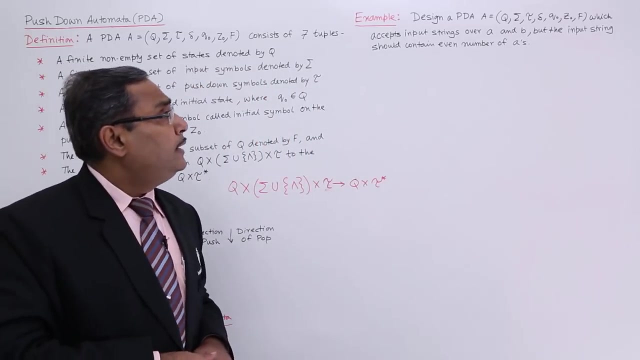 the in the, in this particular push down stored only the top most symbol will be read by this finite control and this is the direction of push and this is my direction of pop. so i think to clear up this particular conception, let us go for one example: see example design. 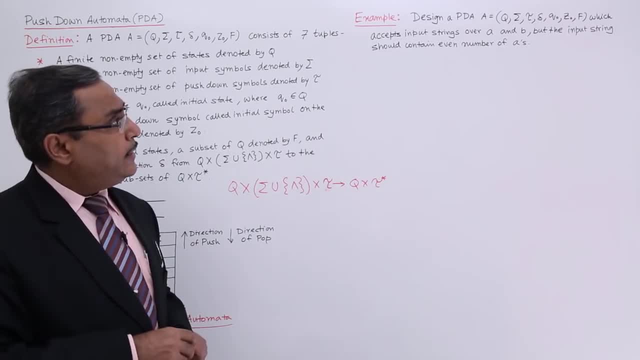 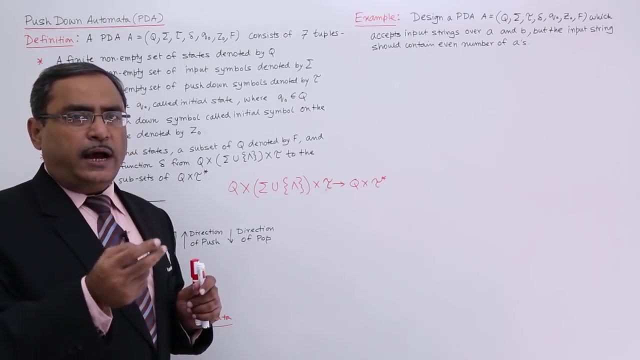 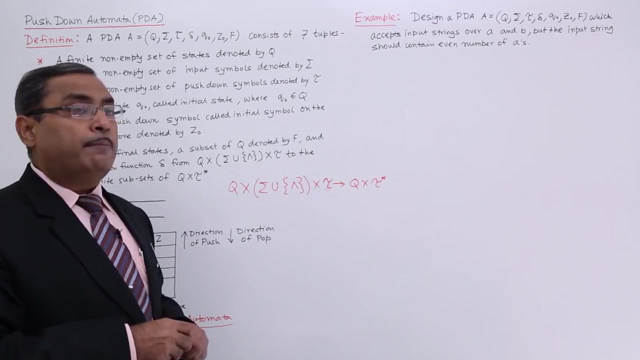 a, pda a. so the pda name is a, q, sigma, tau, delta, q, 0, z 0, f, which accepts input strings over a and b. that means the input string can consist of two symbols, two input alphabets, either a or b or combination of both. okay, but the input string should contain even number of a's. you see, regarding 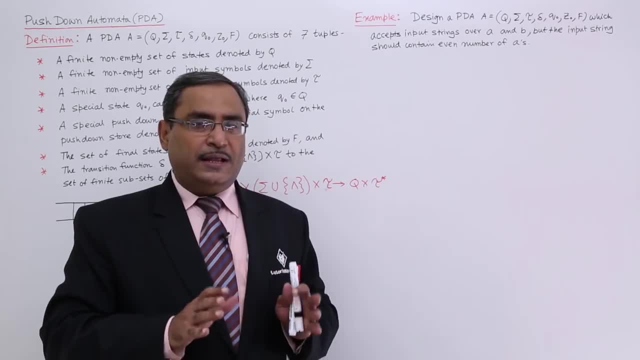 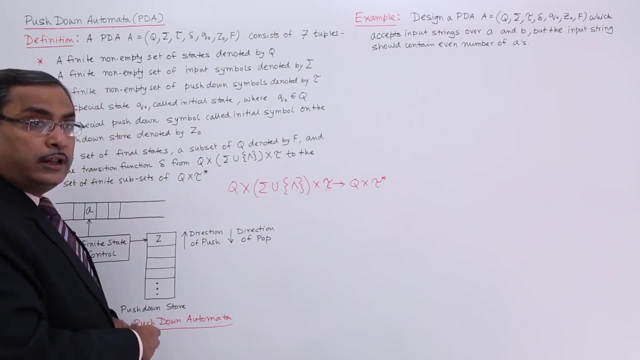 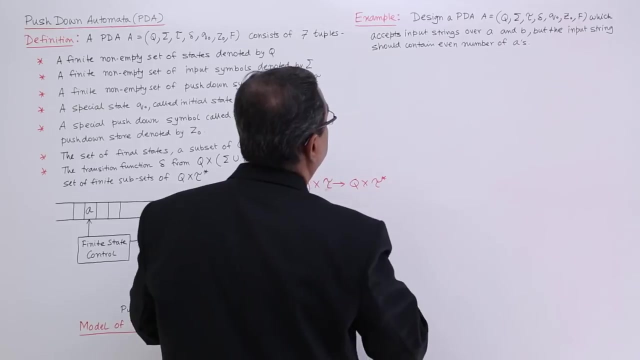 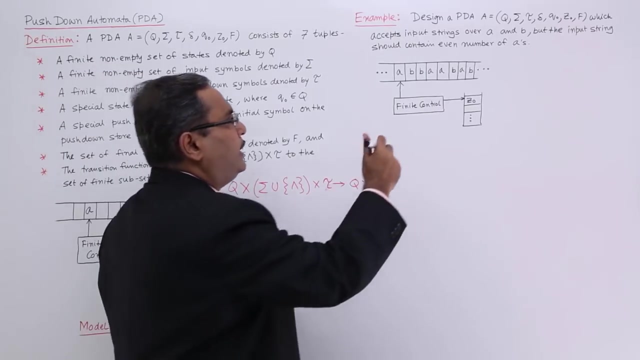 the number of b's, they are remaining silent. that means they are talking about the even number of a's only. so if we draw this particular push down stored model for this particular problem, it will be something like this. so it will be something like this: let us suppose i have taken the string, as i have taken the string. 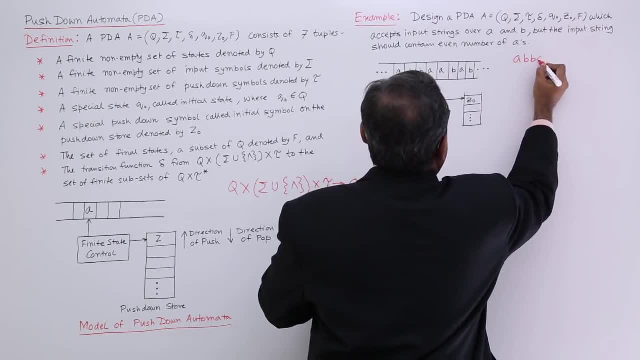 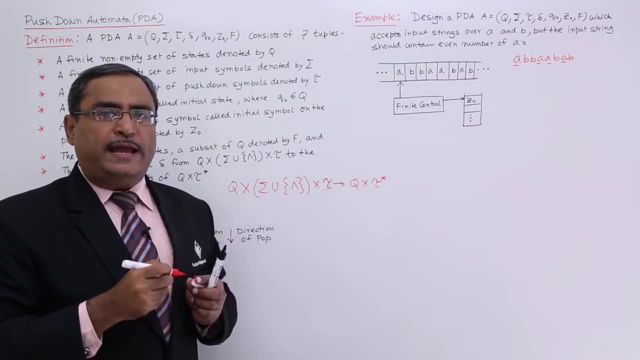 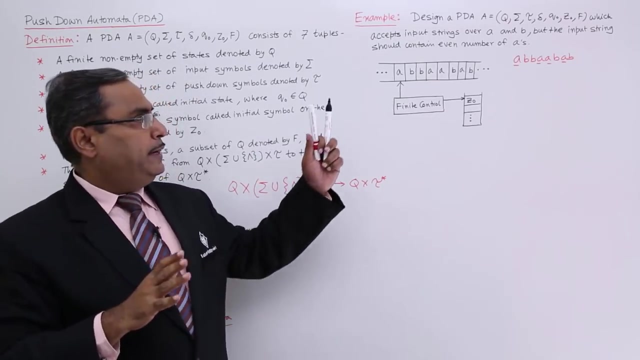 as a, b, b, a, a, b, a, b. so that means one, two, three, four. so i have taken four. number of a's. so that means we are having even number of a's. that means this string will be accepted. it is not mandatory, that always i'll be accepting it. it is not mandatory, that always i'll be accepting it. 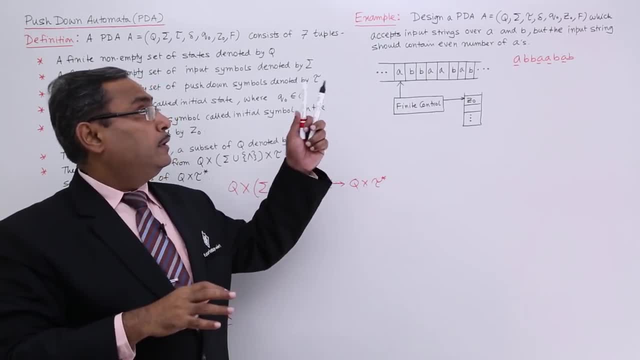 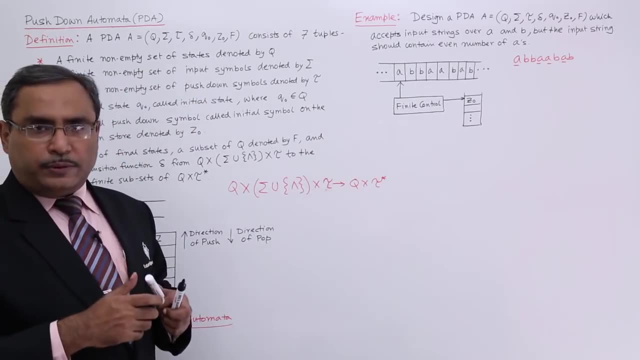 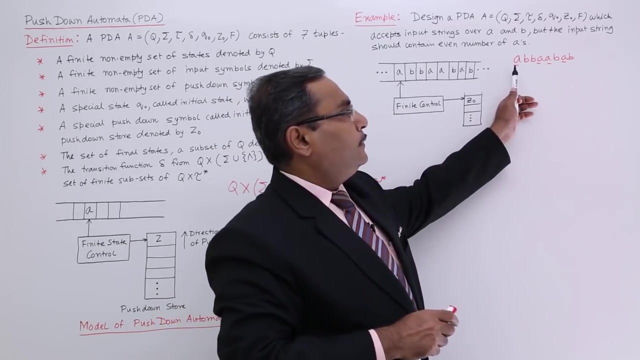 be taking those strings which will be accepted by this um pda. it is not mandatory, but as an example i've taken that one. okay, now see how can i solve this one. see, let us do one thing. if i get a, if i get a, okay, and if the stack top is z 0, then i shall push that a on the top of the stack. 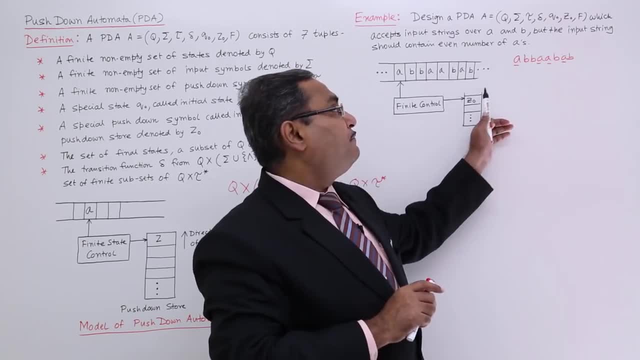 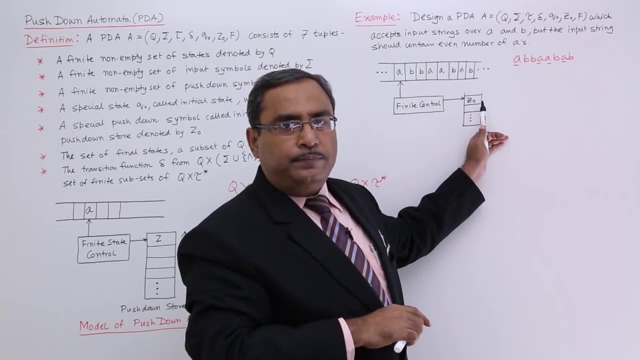 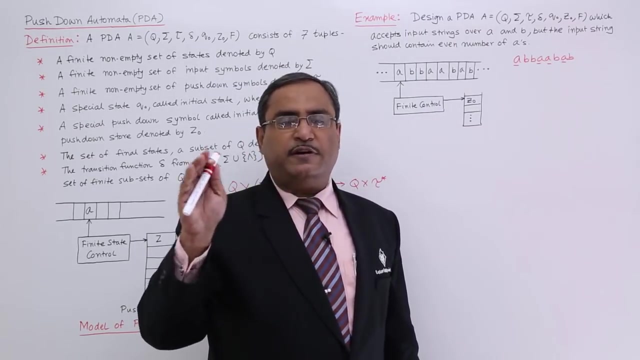 but if i get a and if i find that the stack top is containing a- and if the stack top is containing a, that means prior to that one a was pushed- then i shall pop that one. then what will happen if you have been four a's in a string, not in consecutive fashion, but in some discrete fashions. so first a: 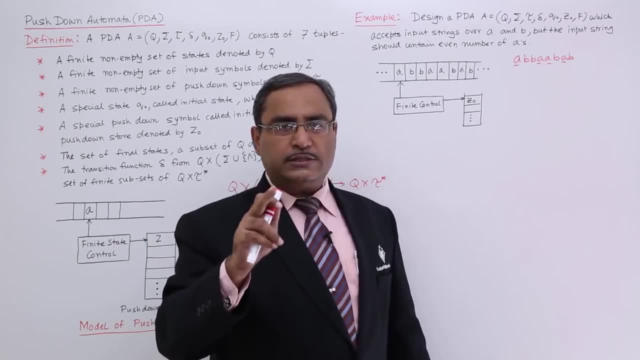 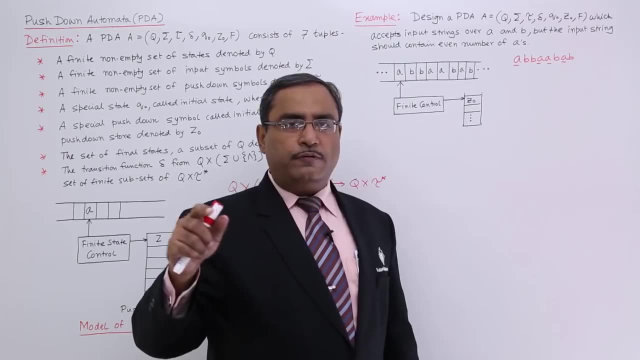 will be pushed. second, for the second a, the a will be popped out from the stack, so stack top will become z 0 again. third a will be pushed. and for the fourth a, it will be popped out from the top of the stack, so again the z 0 will become the top of the push down stored. so if we exhaust, 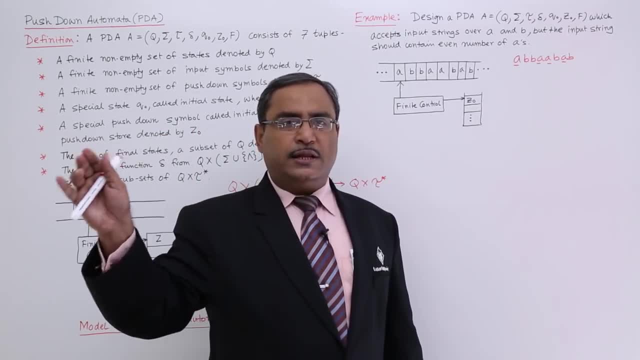 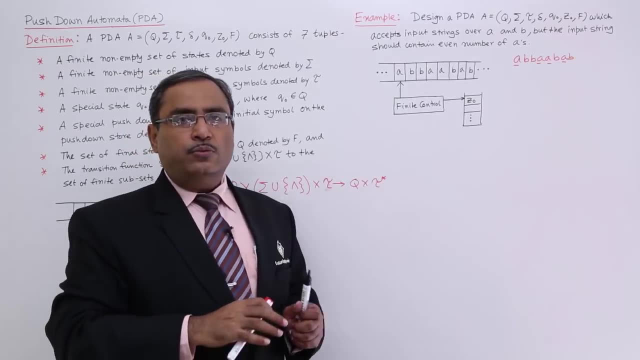 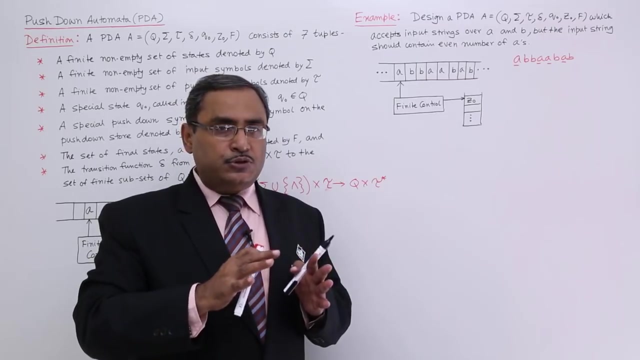 the string and if you find that that z 0 is still on the top of the stack, that will indicate that we had even number of a's and for b's. we are not going to push them, we are not going to pop anything from the top of the stack if you interact with the b. so let us suppose we have. we will be writing. 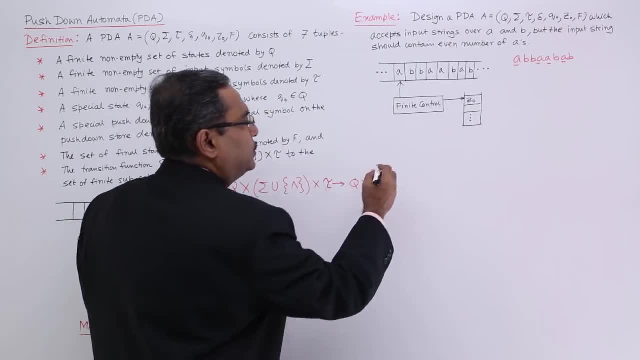 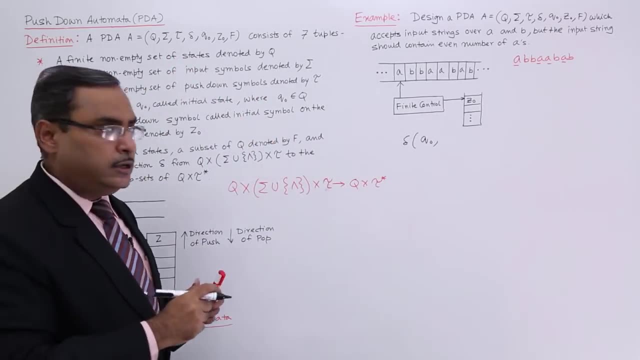 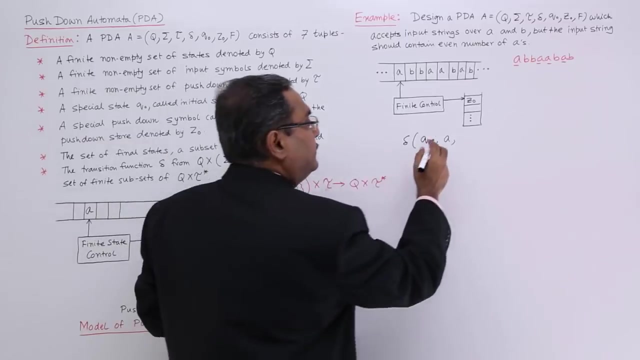 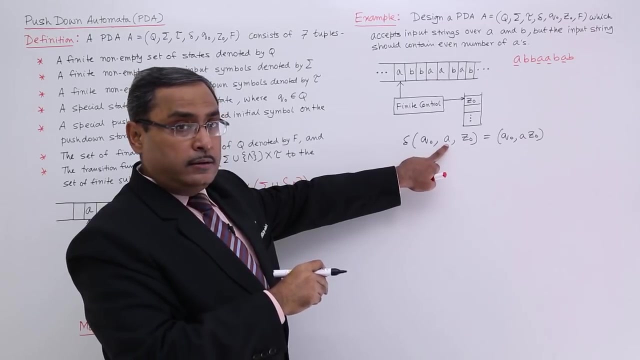 the transitions accordingly. okay, so delta q 0 is the initial state. it has been mentioned that q 0 is the initial state. so if i find a, he means from the input string- if i find a and if i find the top most symbol stack, top is z 0. you see, if i find a where in the input string, if i find myself at the state q 0, 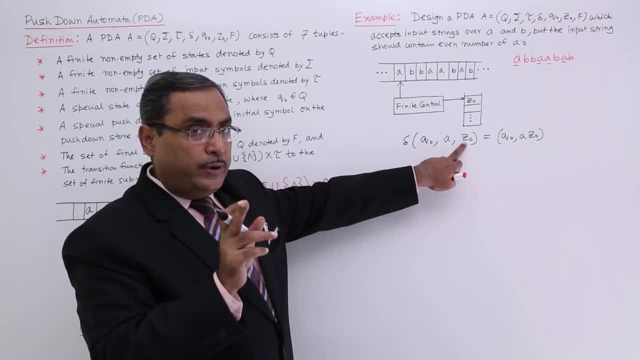 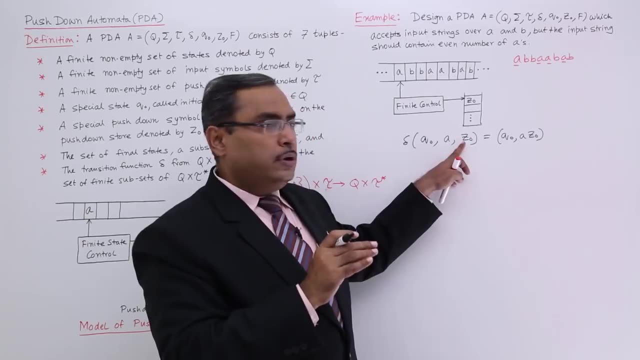 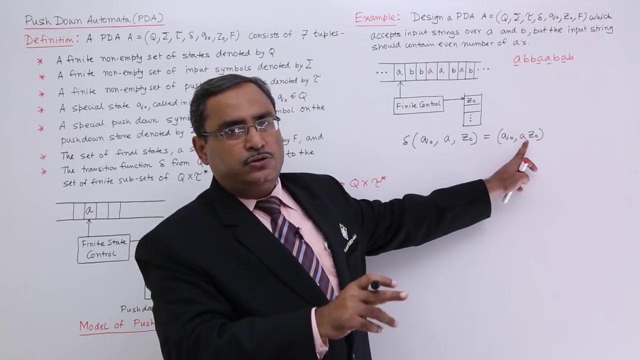 if the stack top symbol is z 0, we had a plan. we did the planning earlier- that i shall push the a on the top of the stack. so here i, here i i have shown z 0, here i am writing a z 0. that means a is at the top and z 0 will be just after that. so that is our convention to write. 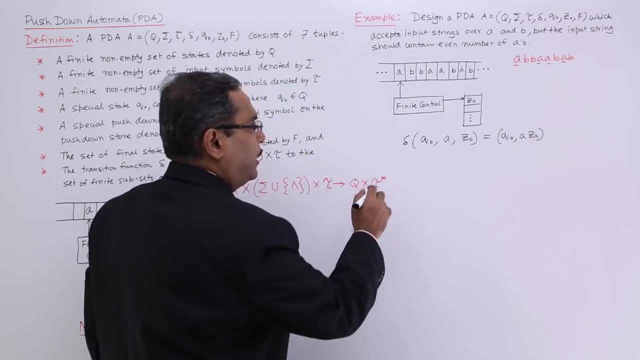 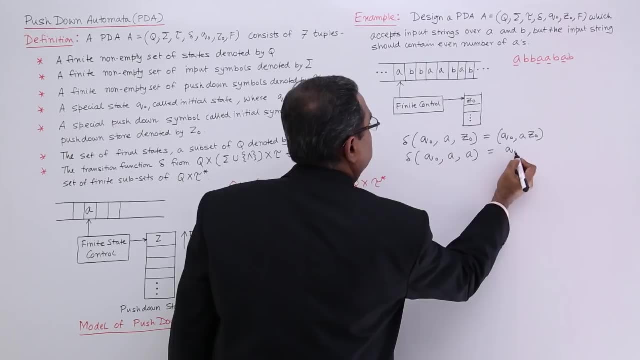 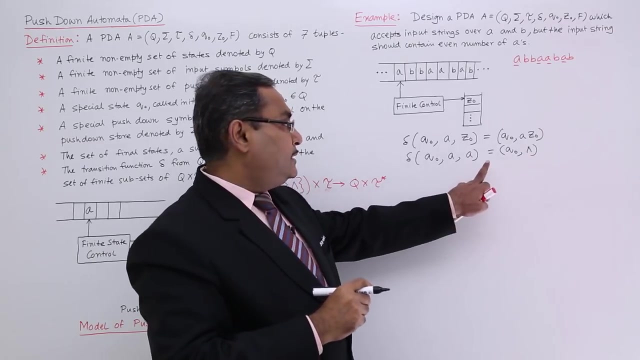 in this way. okay, so q 0, a, z 0. okay, now see. but if we find a and stack top is a, that means i am going to pop that one. here i have shown that one a, but here i have shown kappa means this: a has been. 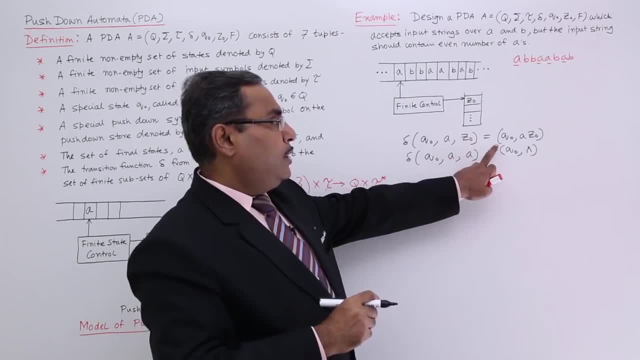 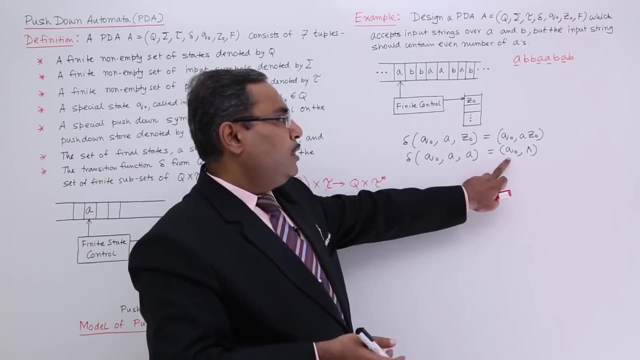 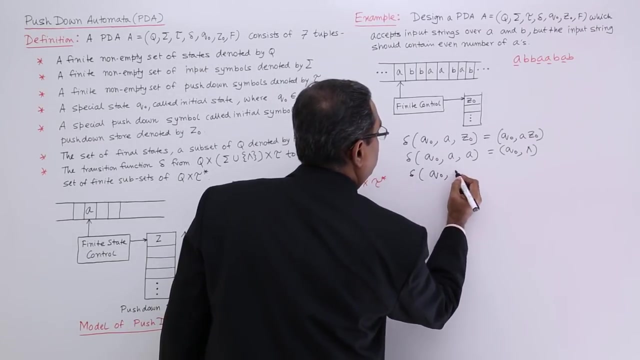 popped out. okay, here i have shown z 0 and here i have shown kappa. means this: a has been popped out. here i have shown a z 0. that means the a has been pushed and z 0 will be just under it. here a has been shown, but here there is no a, so that means a has been popped. delta q 0 b, a will become q 0 a. 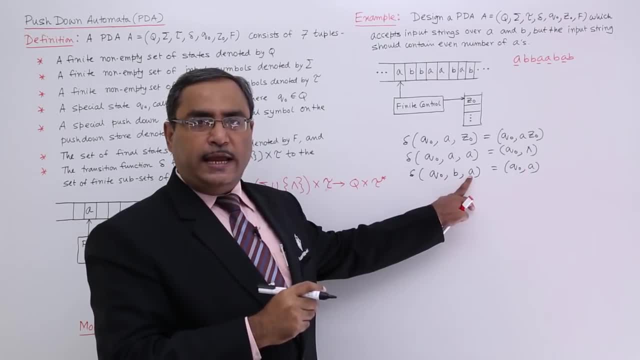 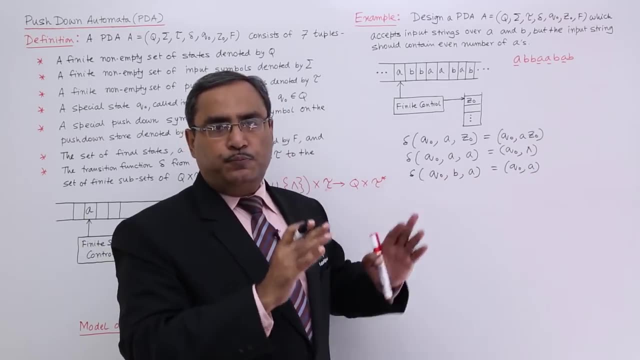 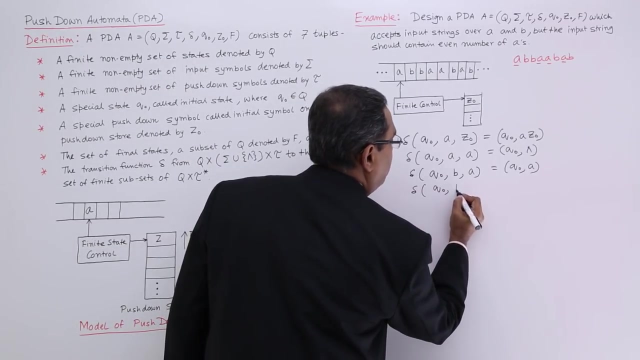 that means if we get b and if the stack top is a, then the a will remain. that means i am not popping out this a. i am just reading this b. i am not pushing it. i am just reading this b. i am not pushing anything. i am not popping anything popping from the push down store. so q 0 b if the stack top. 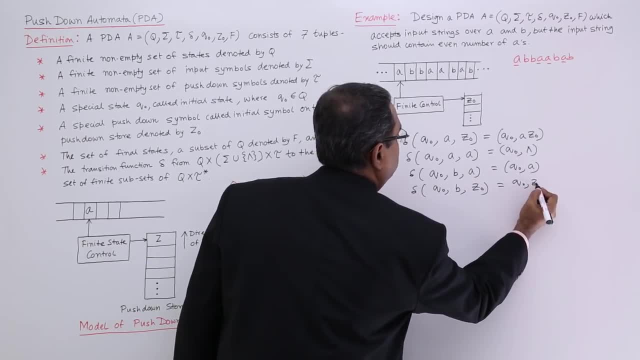 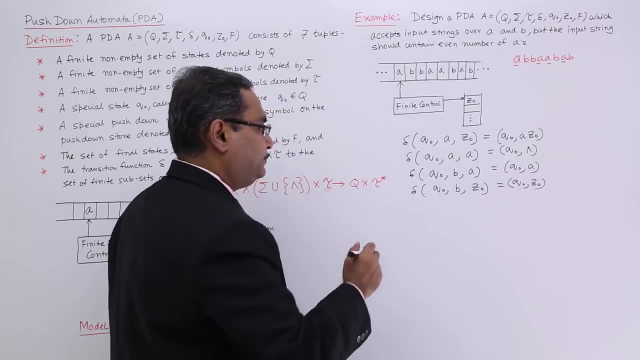 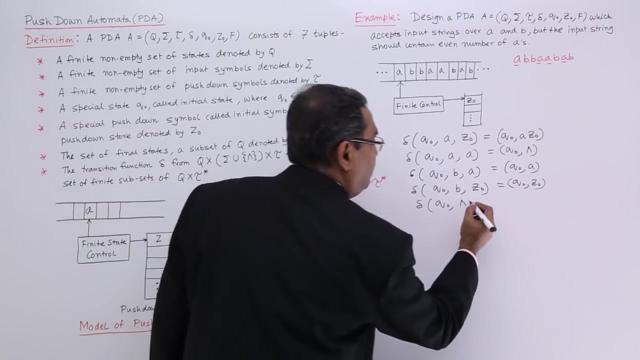 is z 0 in that case, then also the stack top z 0 will be there. so that is the other condition. okay, now the last one: if i am at the state q 0 and the if, if the input has got exhausted and if my stack. 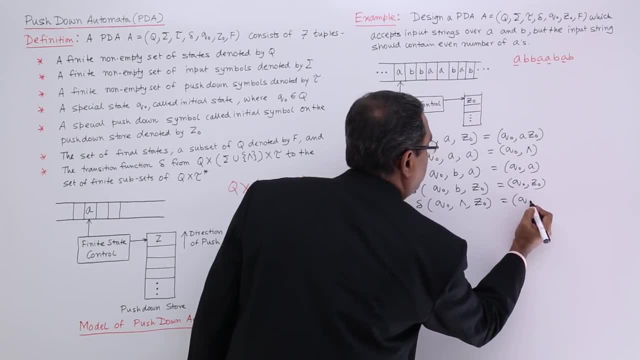 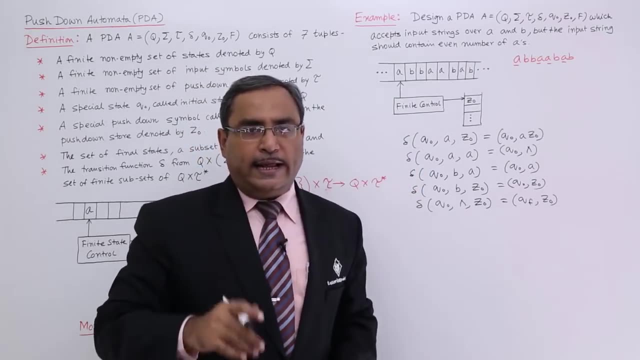 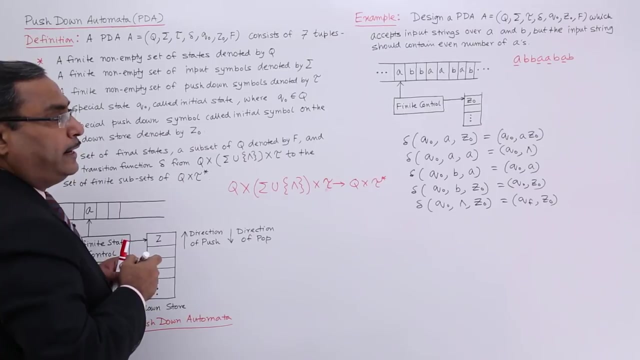 top symbol is z 0, then i shall go to the q f, the final state, and then my stack top is z 0. so, reaching to the final state, the string will get accepted. okay, now let me explain each and everything. what about the q here? if i want to, 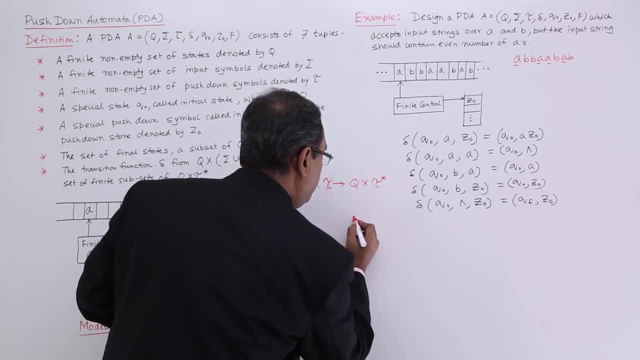 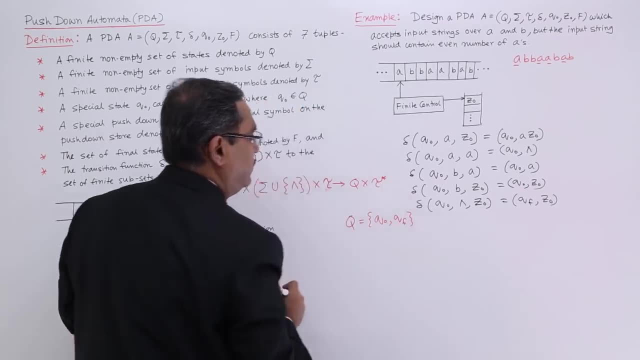 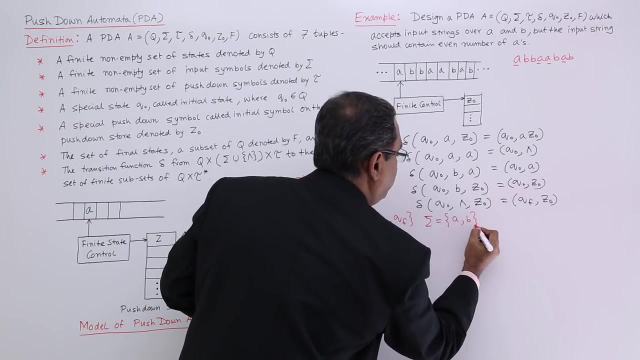 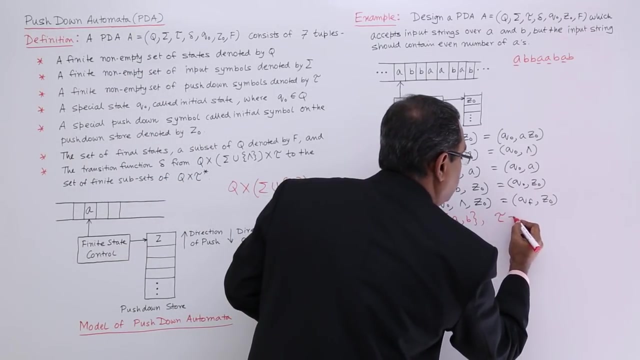 write q, so i am writing q here. see what is the q? here we are having q 0 and q f. okay, so q has been defined. what about the sigma? sigma is nothing but a and b input symbols, okay. what about the tau? tau means push down, store symbols, obviously tau. 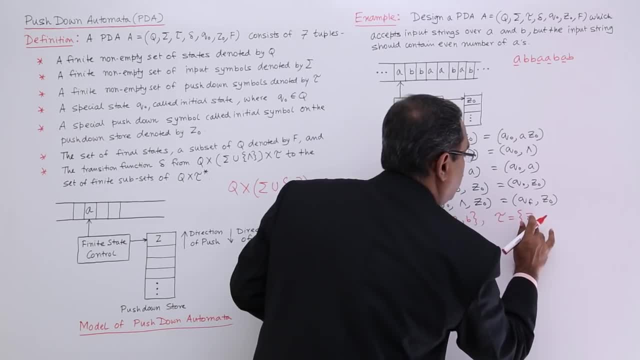 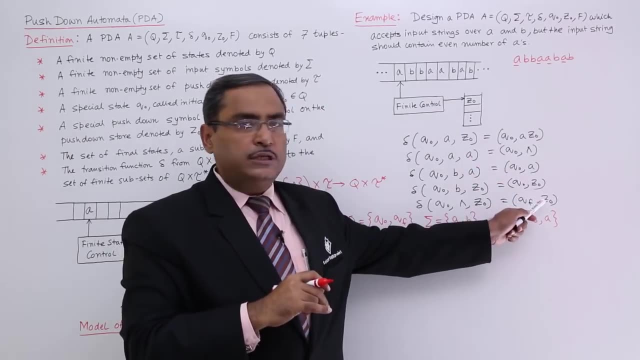 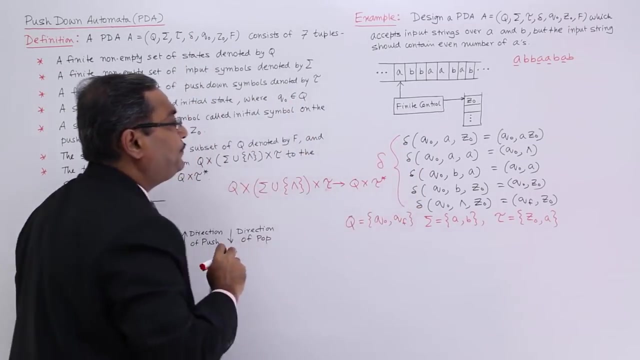 will be consisting of z 0 and a. don't consider b here, because you didn't push b on this particular push down store, so b will not be coming. so what about this delta? delta is this one. so this is my delta. okay, what about the q 0? q 0 is initial state. 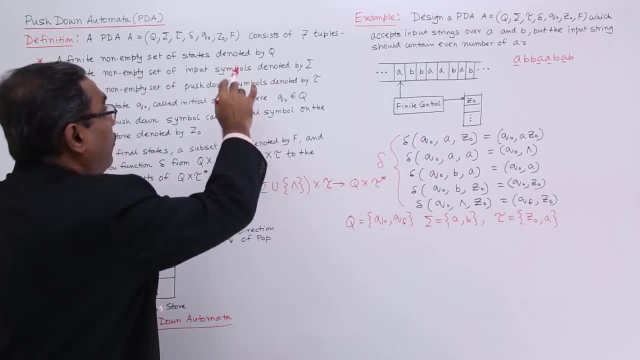 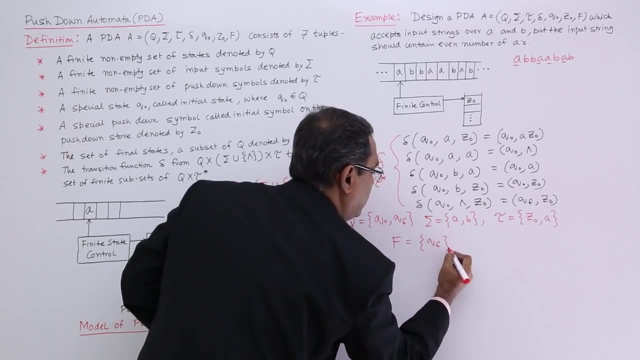 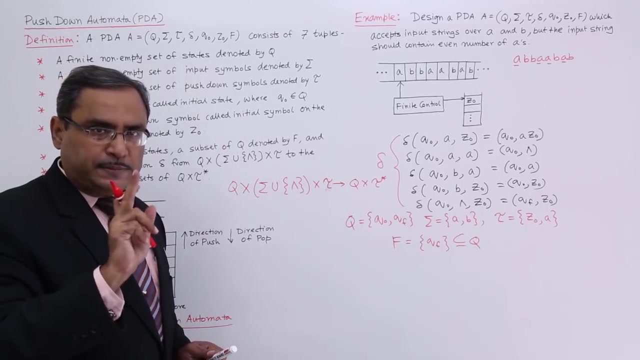 what about the z 0? z 0 is my stack top symbol. what about the f? what about the f f? here is q, f, which is a subset of capital. q done. so i have explained each and everything. now let me explain the last one. see, look at the q. so what is the first component you are having? what is the first? 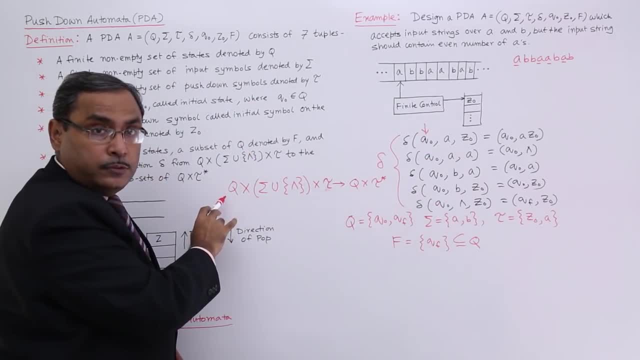 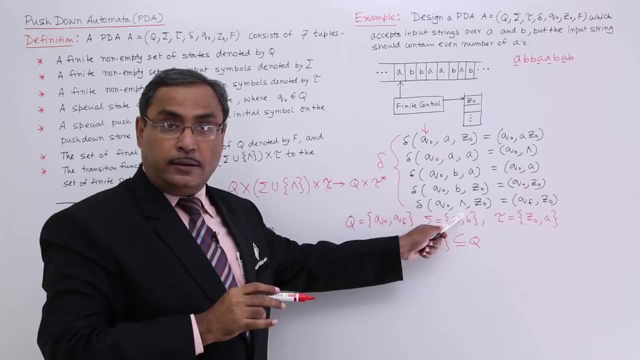 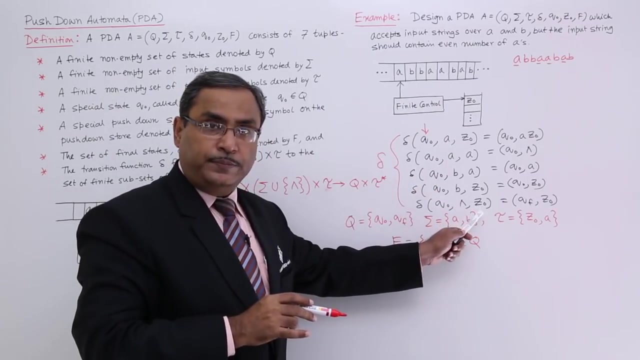 component. you are having one of the members of capital q. good, and then which? which is coming in addition, either sigma or kappa. you see either sigma or kappa, either a or b or kappa. what about the third argument? see, they are nothing but the push down store element. what are the push down? 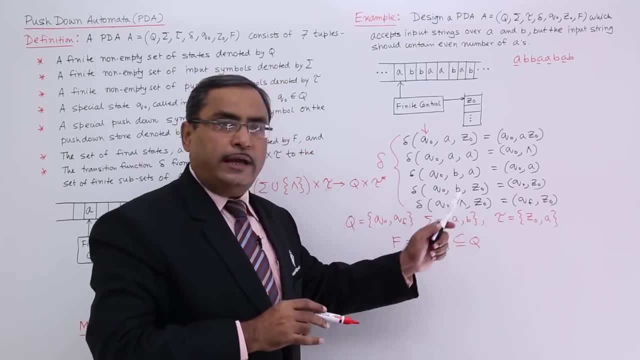 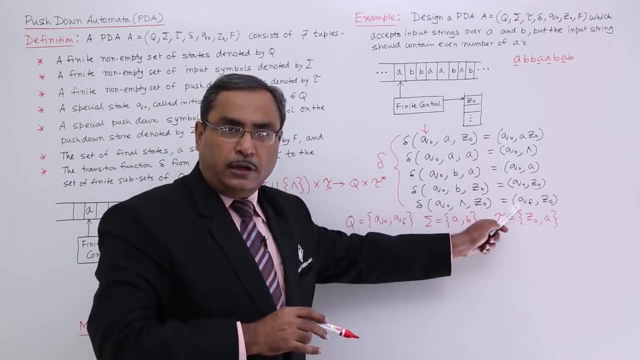 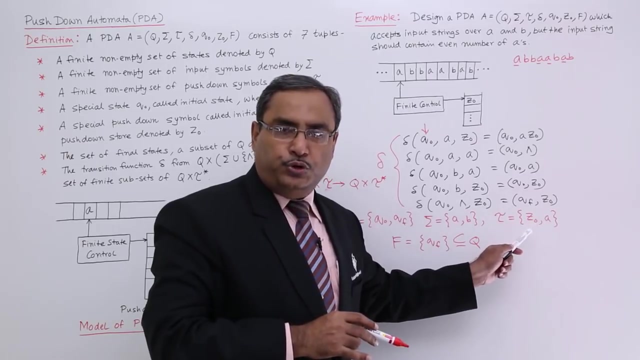 store elements z, 0 or a. so either z 0 or a is coming. so now it maps to q. what is q? that is one of the states of capital. q. cross condition product: tau star, tau star means what means the string consisting of this push down store symbols. you see we are having tau star, tau star can. 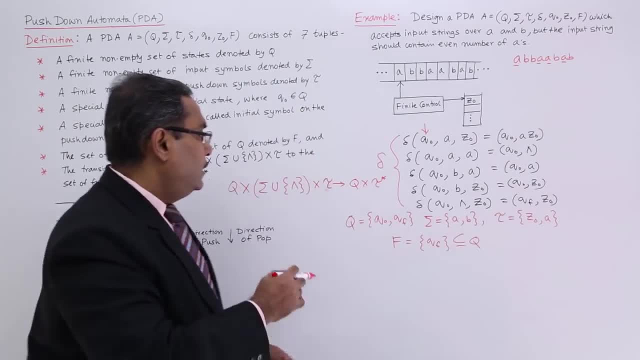 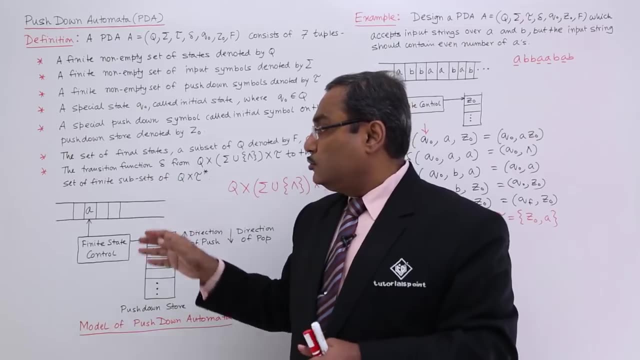 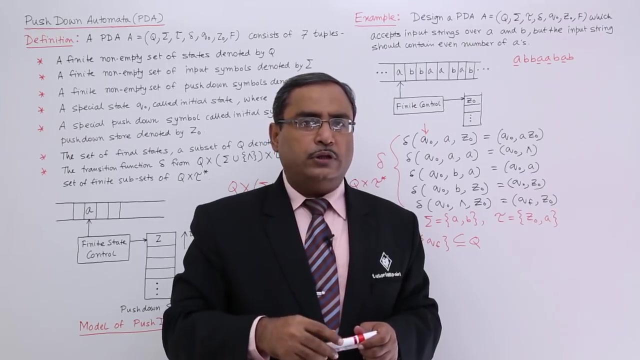 be also kappa. so in this way you see the thing has got explained. so i think how to define one push down automata and how to work with that, to some extent you have got the idea in the next videos in this particular section we are have. we are going to solve so many problems on this push down.